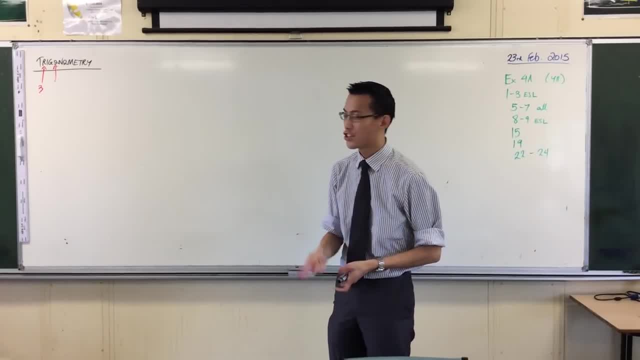 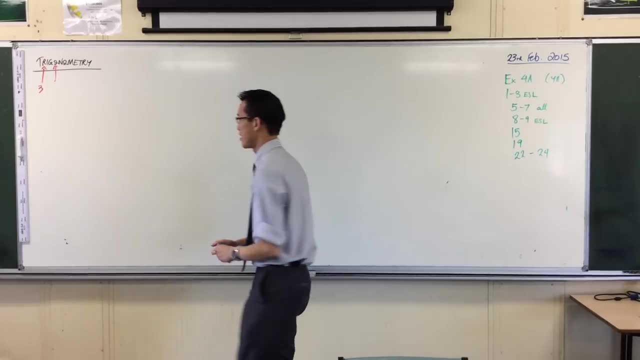 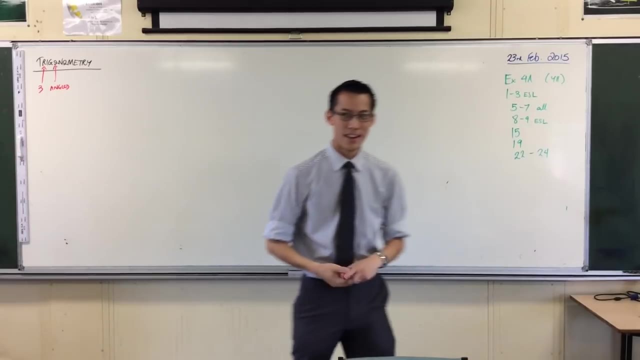 It means angles. angles just like polygons, right? I know we're used to thinking of that as many-sided, but actually it means many angles. So a trigon is a three-angled shape. Now, when you see, you know o-metry, on there, o-metry, there's a few different like o- sort of suffixes. you can see. 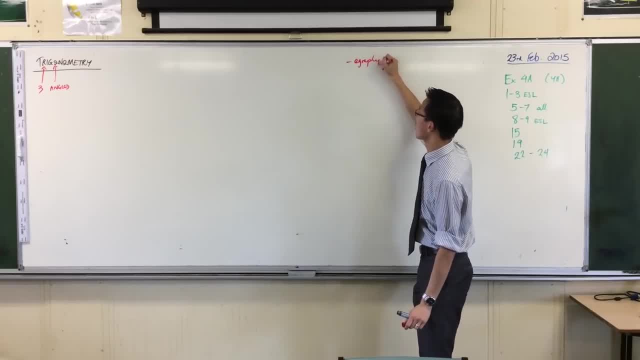 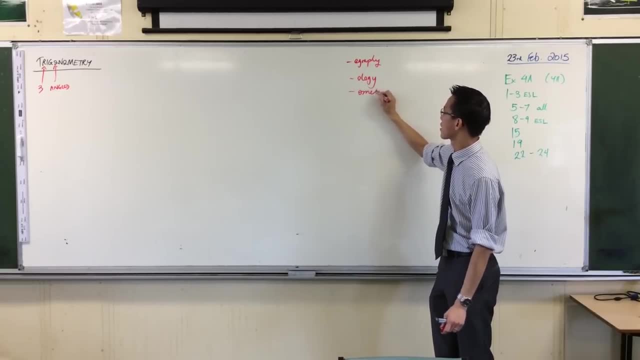 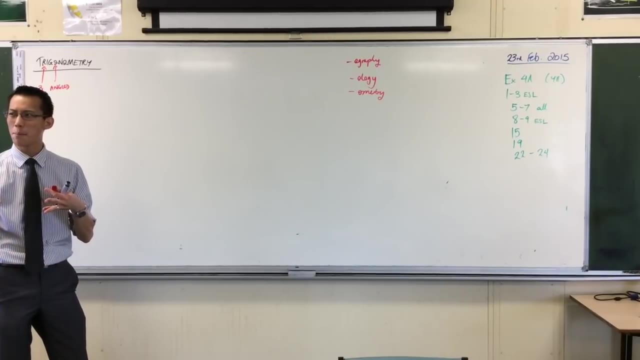 Like there's o-graphy, like geography, right. There's ology, like topology, and then there's o-metry. What is that? What does this mean? We don't tend to see this in many contexts. There's optometry. 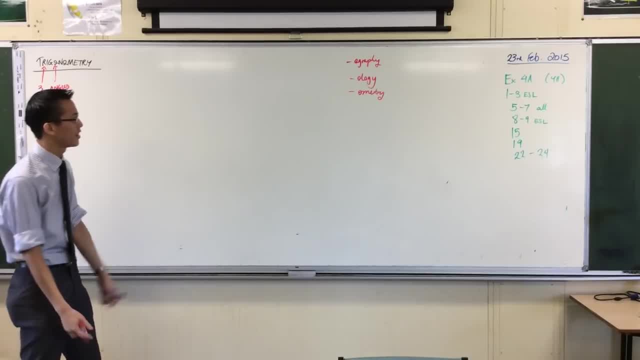 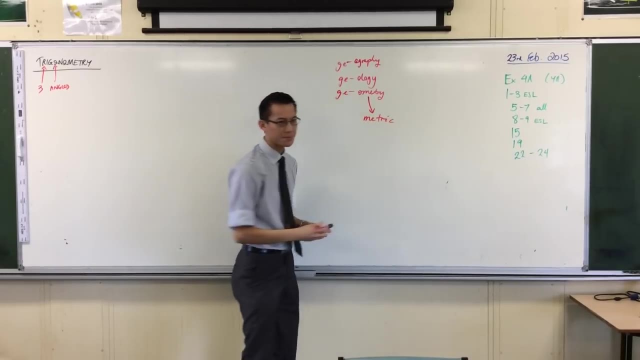 Optometry. so it's kind of: what's that about? There's geometry. You can put geo in front of any of these. by the way, Geometry, geology- It may help if you know another word that we use which comes from the same basis, namely metric. 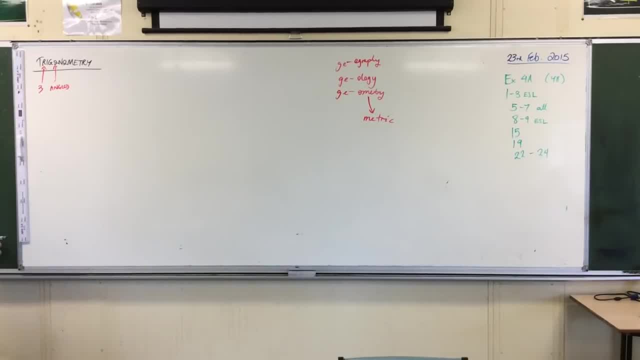 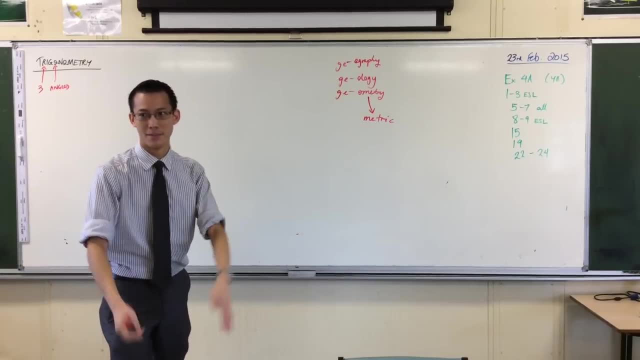 So metric is about measurements. Okay. If I say you know what are the metrics on x, y, z, Okay. Or if we talk about the metric system, it literally means the system that you use to measure stuff. Okay. 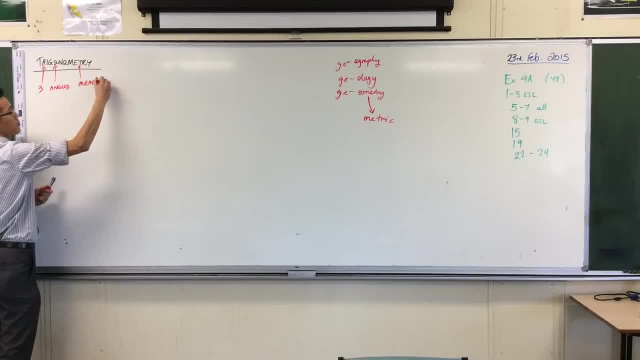 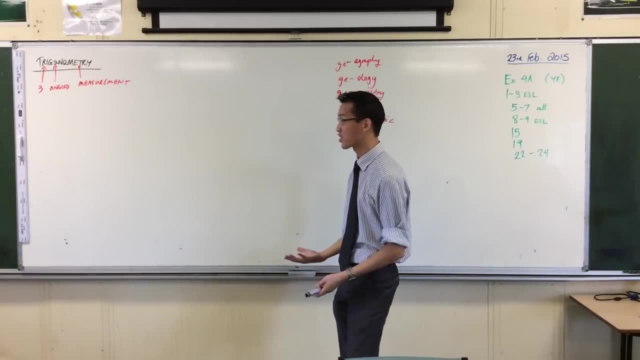 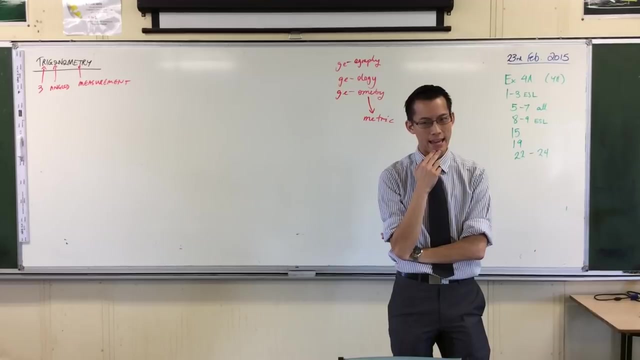 So this is about measurement, Measurement. So essentially this means: okay, it's about measuring triangles, And that's kind of all the name implies. This is where trigonometry begins, But it's not where trigonometry ends. In fact, trigonometry kind of has a way of getting into everything. 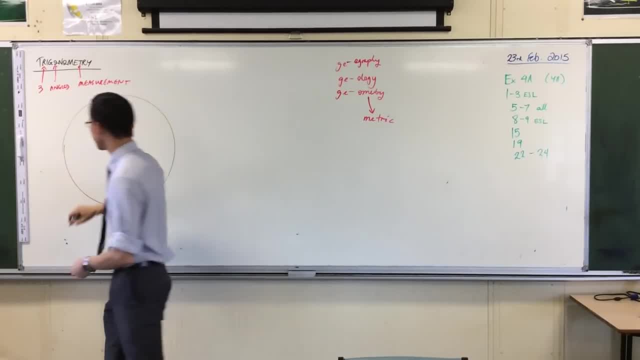 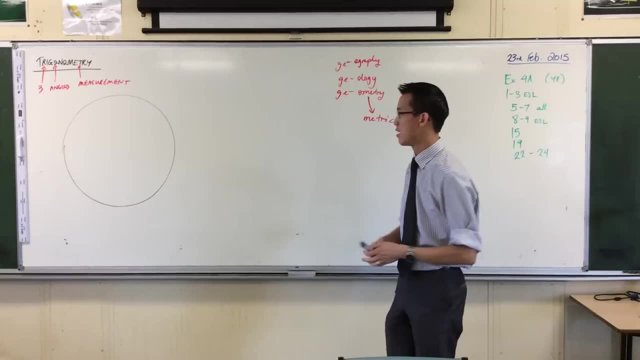 Example: if you have a think about anything that operates in cycles, right. Anything that's periodic and it repeats itself over and over again, right. When you have something that's periodic and it's repetitive, we have a name for this that's based on this shape. 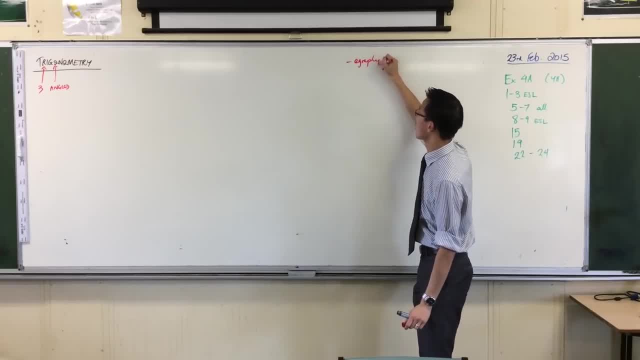 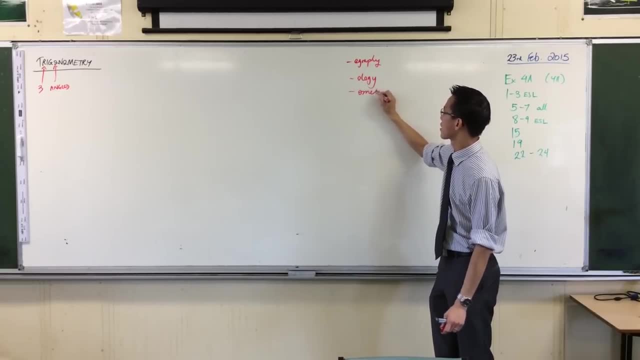 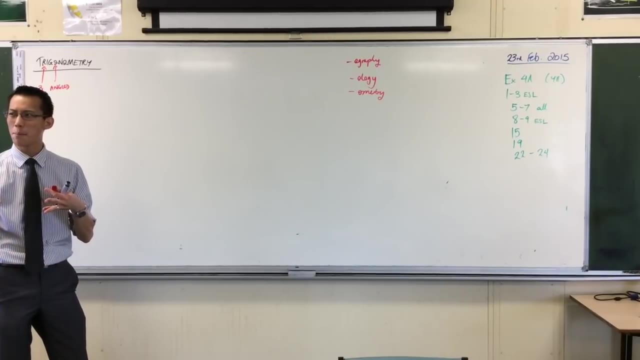 Like there's o-graphy, like geography, right. There's ology, like topology, and then there's o-metry. What is that? What does this mean? We don't tend to see this in many contexts. There's optometry. 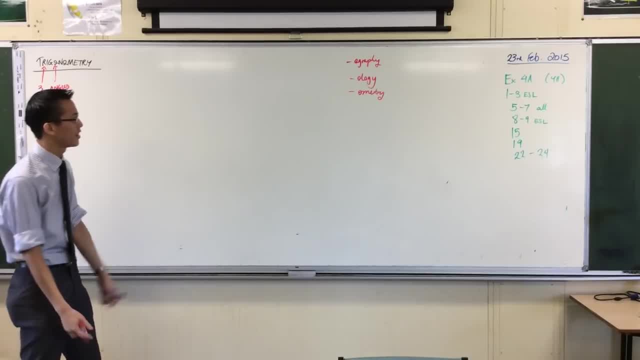 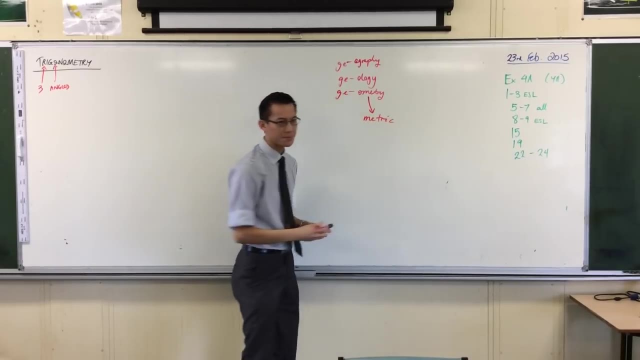 Optometry. so it's kind of: what's that about? There's geometry. You can put geo in front of any of these. by the way, Geometry, geology- It may help if you know another word that we use which comes from the same basis, namely metric. 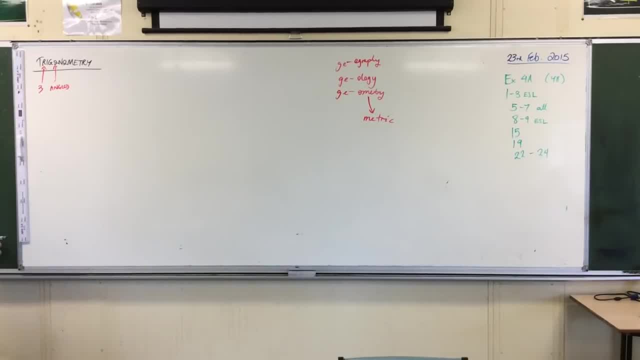 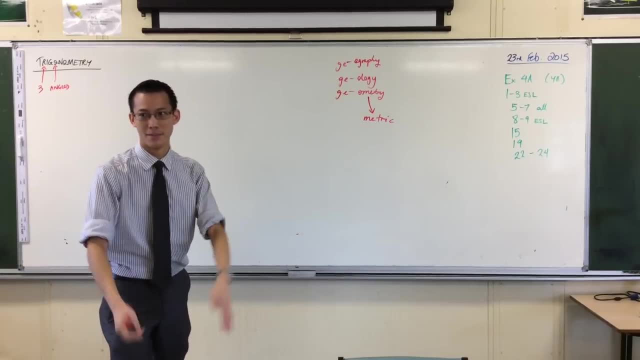 So metric is about measurements. Okay. If I say you know what are the metrics on x, y, z, Okay. Or if we talk about the metric system, it literally means the system that you use to measure stuff. Okay. 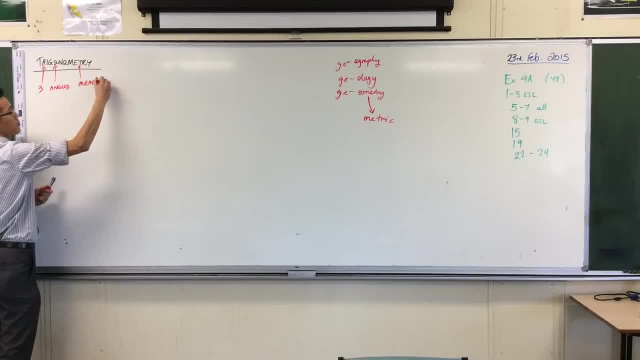 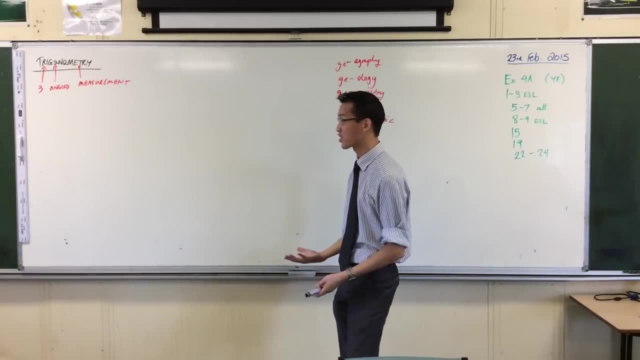 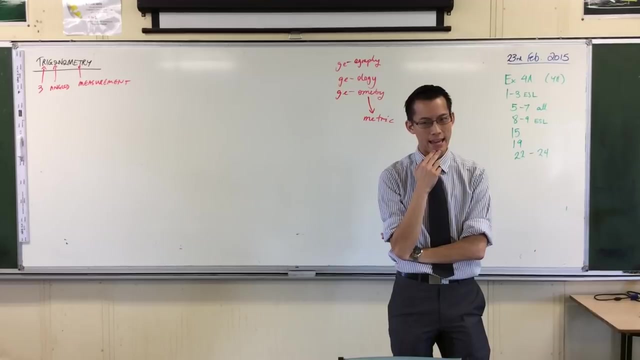 So this is about measurement, Measurement. So essentially this means: okay, it's about measuring triangles, And that's kind of all the name implies. This is where trigonometry begins, But it's not where trigonometry ends. In fact, trigonometry kind of has a way of getting into everything. 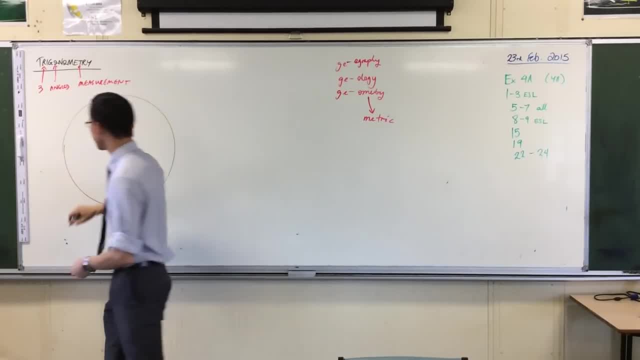 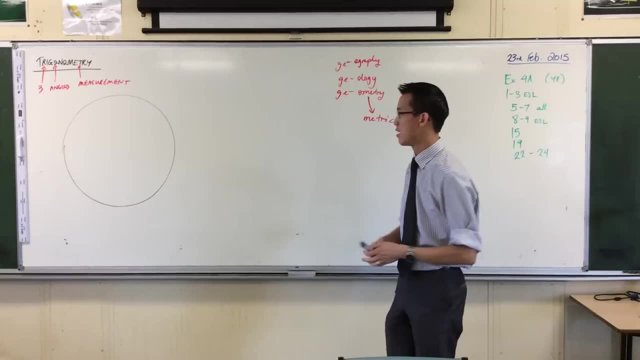 Example: if you have a think about anything that operates in cycles, right. Anything that's periodic and it repeats itself over and over again, right. When you have something that's periodic and it's repetitive, we have a name for this that's based on this shape. 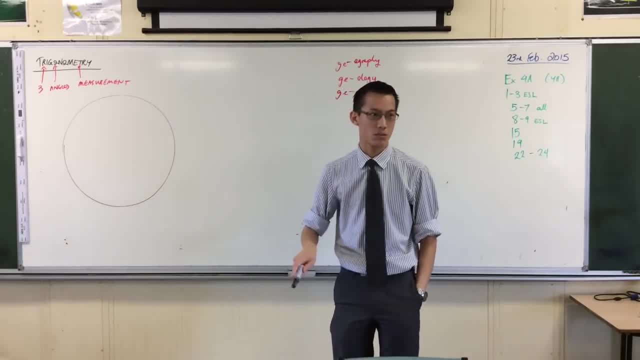 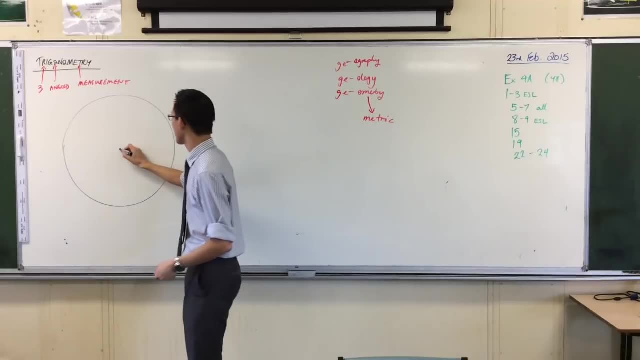 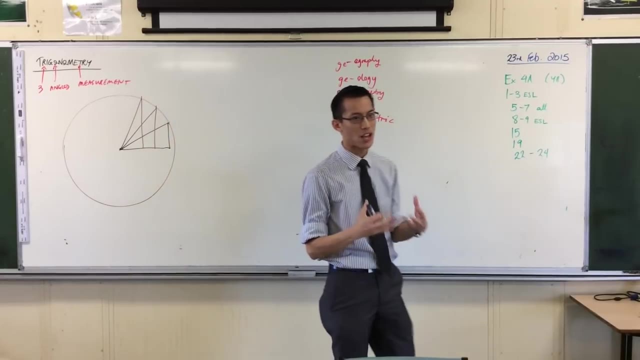 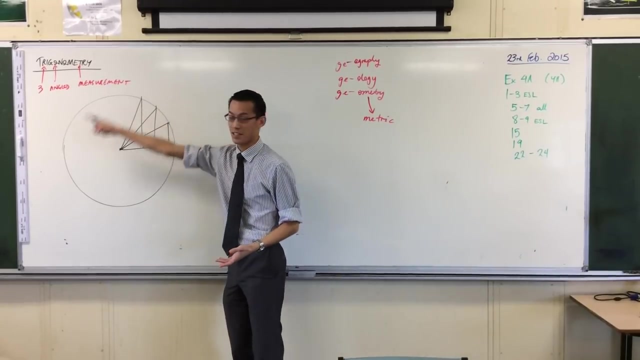 We call it cyclic, right? Like? it goes around in circles. Well, every circle- If I want to actually do any measurement of what's happening in this circle- every circle is actually built up of a series of triangles, right? So anywhere you find cyclic things, periodic things, things that happen over and over again, despite the fact that it doesn't look like it has to do with triangles. you get trigonometry in there, right? 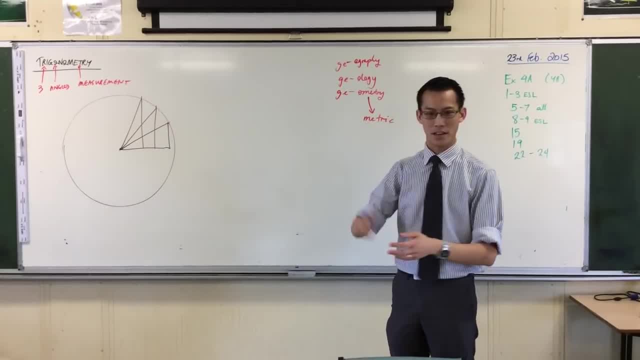 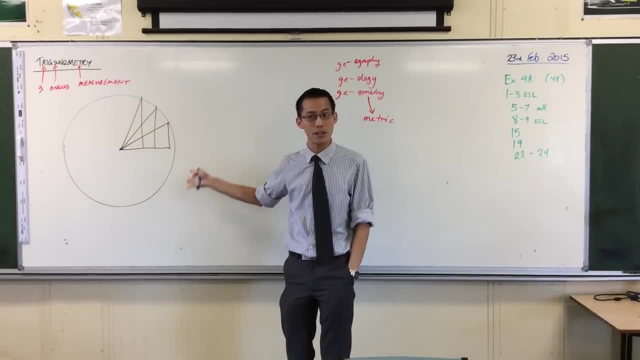 So when we move on to simple harmonic motion, which is kind of things moving up and down or left and right or round and round, it's all in terms of trigonometric functions, right? So that's in terms of things that go round and round or oscillate. 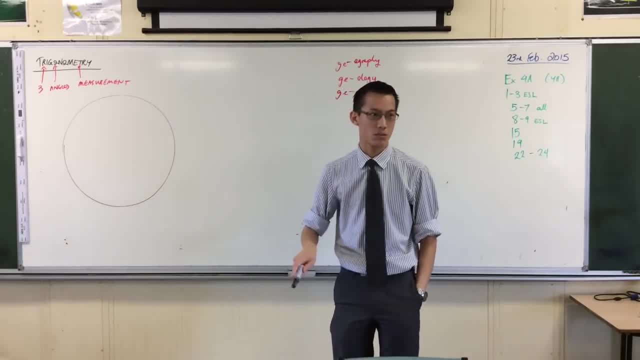 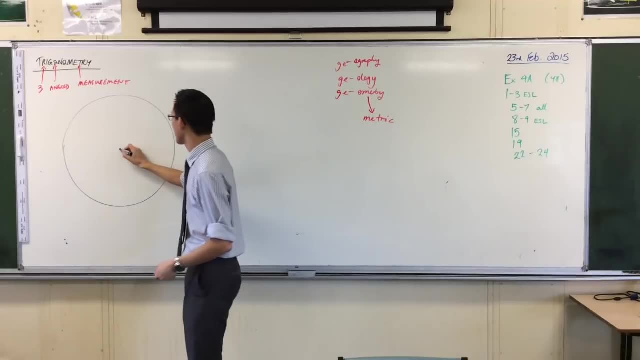 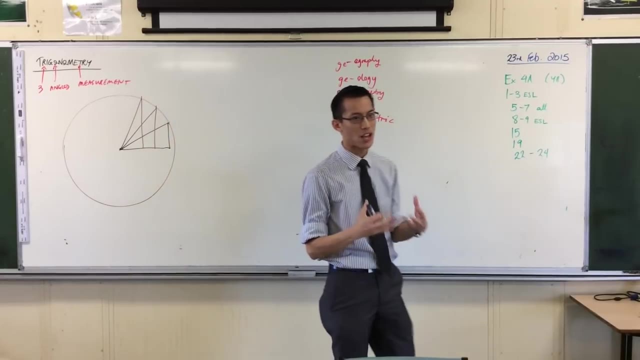 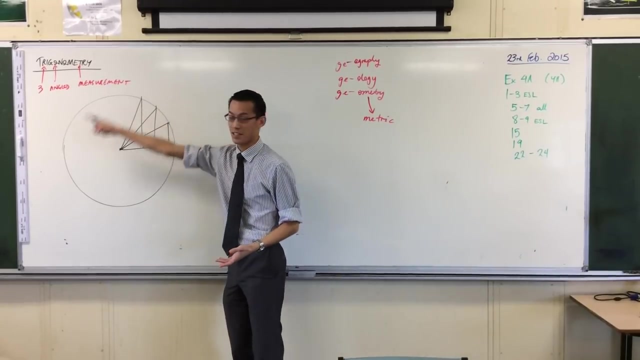 We call it cyclic, right? Like? it goes around in circles. Well, every circle- If I want to actually do any measurement of what's happening in this circle- every circle is actually built up of a series of triangles, right? So anywhere you find cyclic things, periodic things, things that happen over and over again, despite the fact that it doesn't look like it has to do with triangles. you get trigonometry in there, right? 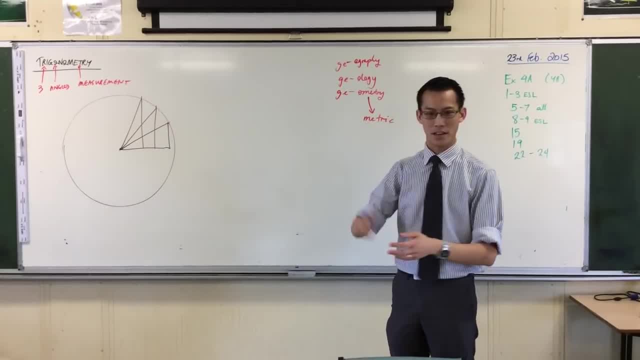 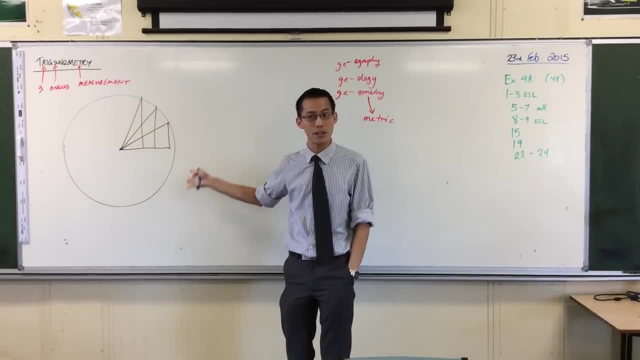 So when we move on to simple harmonic motion, which is kind of things moving up and down or left and right or round and round, it's all in terms of trigonometric functions, right? So that's in terms of things that go round and round or oscillate. 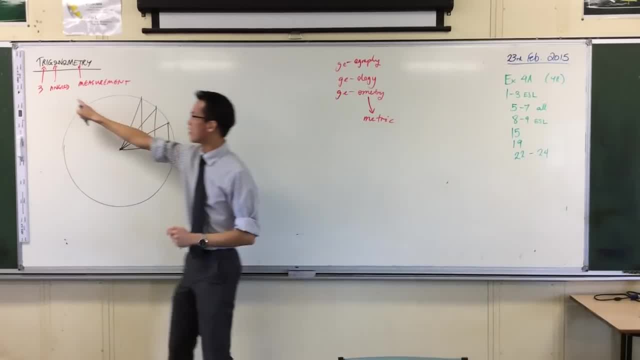 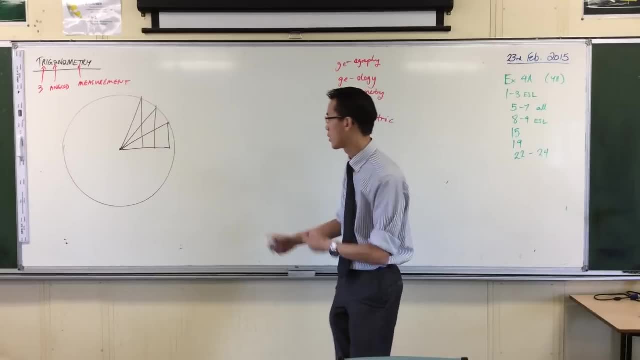 There's one other quick example, Because you know it's about angle measurement. Anytime anything happens in angles, trigonometry will be involved. right Quick example: Thinking of simple harmonic motion. the next big application of trigonometry that you find in the Extension 1 course is what we call projectile motion. 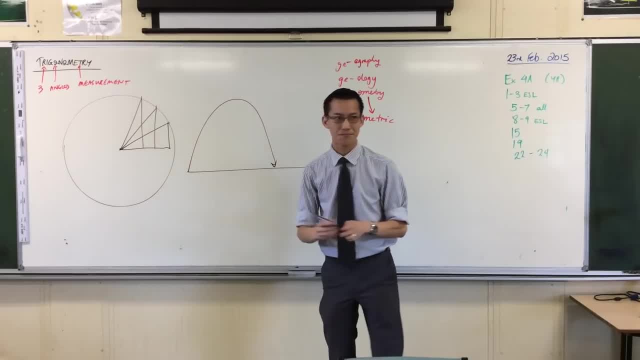 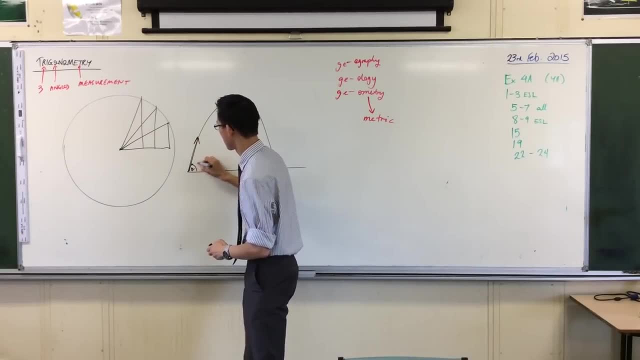 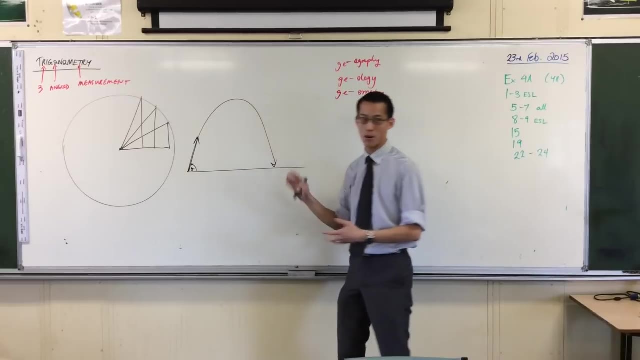 So if you have an object right and you fire it at a certain angle, like this, at a certain velocity and so on, right the way to understand what's going on here, like how high it'll go and how far it'll go, all those kinds of things are understood in terms of trigonometry, right? 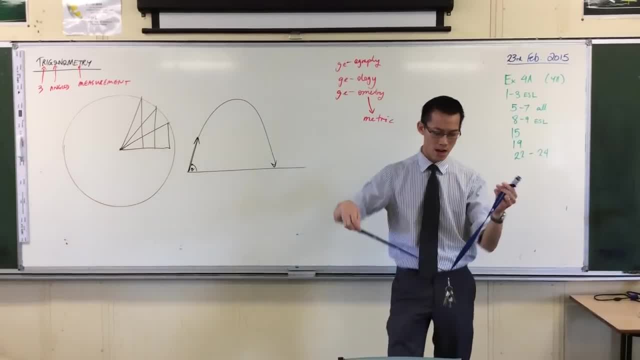 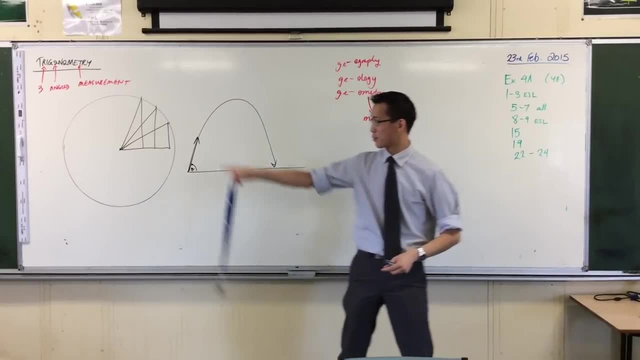 Even things like, if you want to go a little bit further in the. this is all Extension 1, in the Extension 2 topic called circular motion, we look at things that we'll just go back to the circle. we look at things that do this. 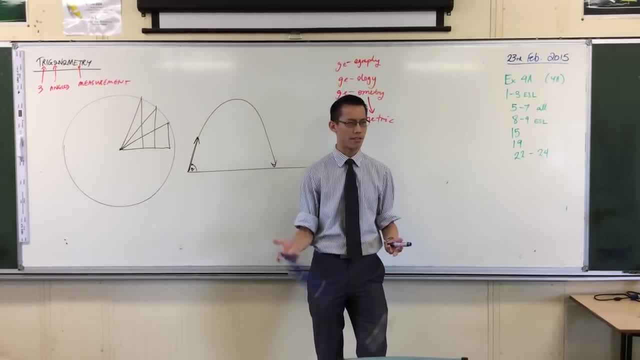 They go round and round and round. Now, clearly, you can sort of think about this as like a: well, it's a cycle of kinds, right, But it's not what we call simple harmonic motion. Simple harmonic motion is just in one dimension. 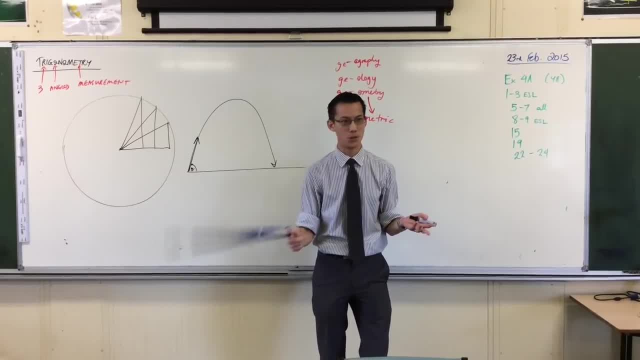 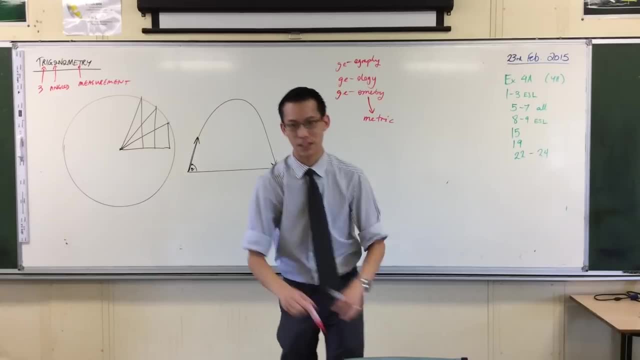 So it's up, down or left, right, Whereas this is in two dimensions. And now you're feeling very, very sleepy. Now hold on. What's happening to this thing, right? If I use my conveniently drawn circle here, 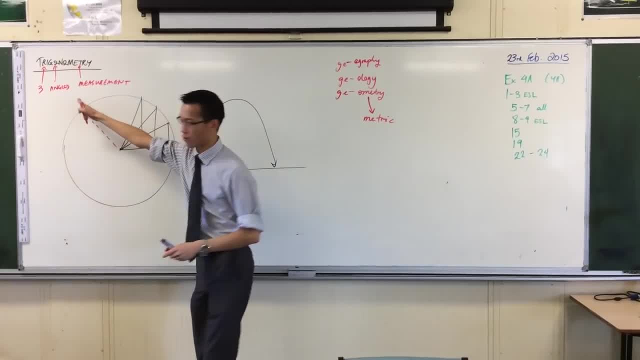 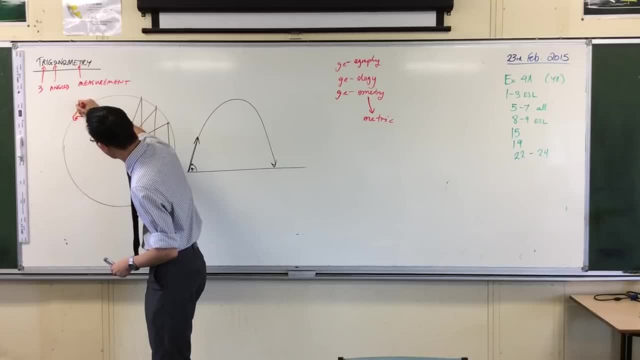 I've got my um, I've got my string holding something to a center of motion. there's my finger in the middle, right, And then you've got the keys flying around there, right? That's a beautiful diagram, okay. 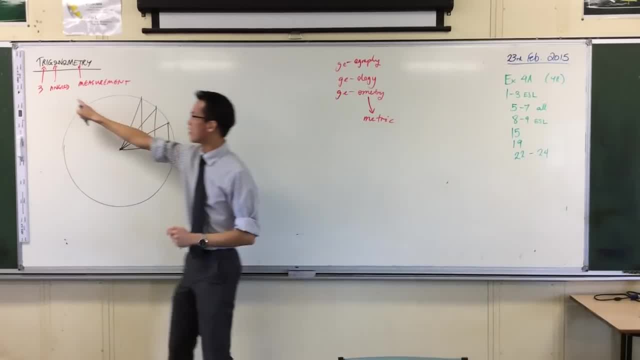 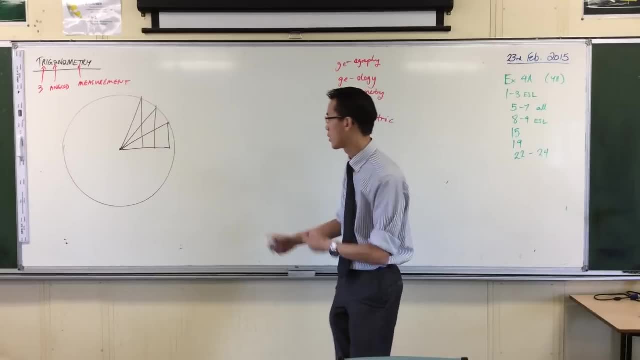 There's one other quick example, Because you know it's about angle measurement. Anytime anything happens in angles, trigonometry will be involved. right Quick example: Thinking of simple harmonic motion. the next big application of trigonometry that you find in the Extension 1 course is what we call projectile motion. 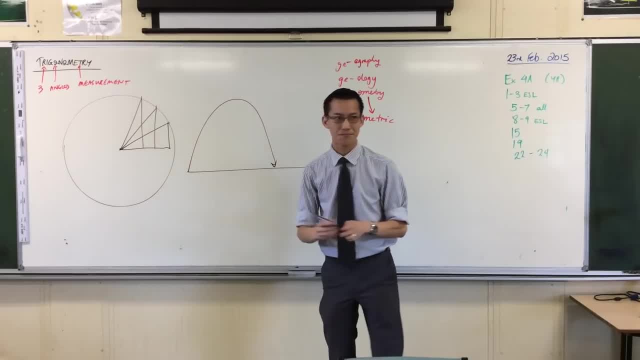 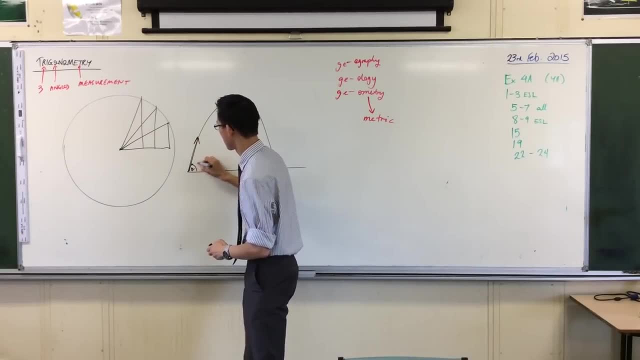 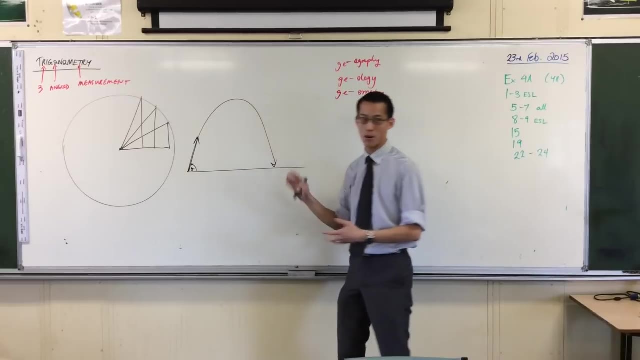 So if you have an object right and you fire it at a certain angle, like this, at a certain velocity and so on, right the way to understand what's going on here, like how high it'll go and how far it'll go, all those kinds of things are understood in terms of trigonometry, right? 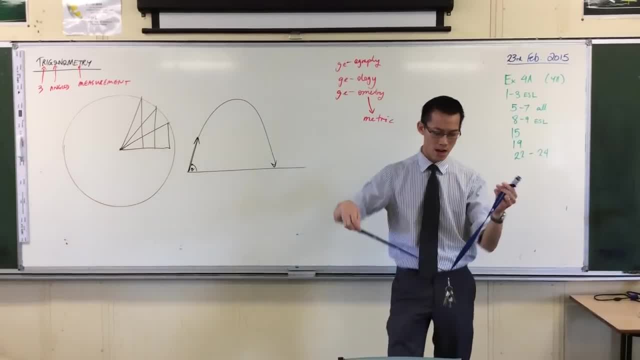 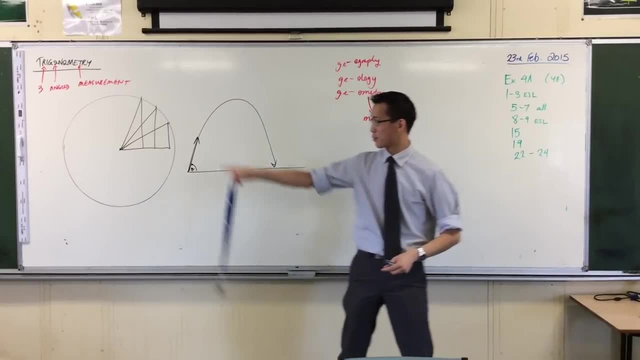 Even things like, if you want to go a little bit further in the. this is all Extension 1, in the Extension 2 topic called circular motion, we look at things that we'll just go back to the circle. we look at things that do this. 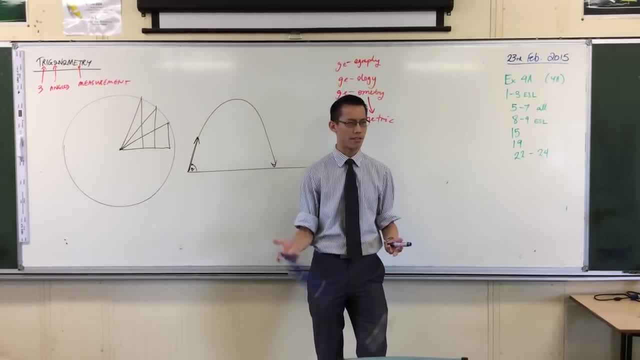 They go round and round and round. Now, clearly, you can sort of think about this as like a: well, it's a cycle of kinds, right, But it's not what we call simple harmonic motion. Simple harmonic motion is just in one dimension. 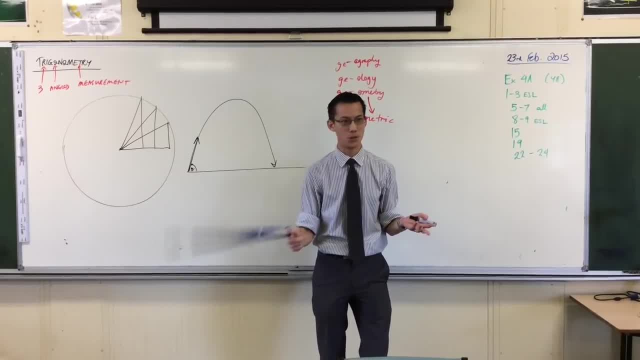 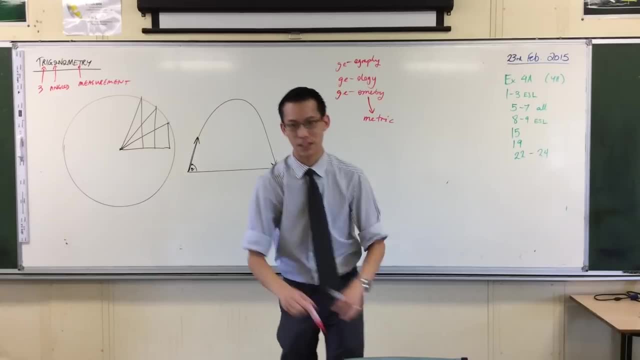 So it's up, down or left, right, Whereas this is in two dimensions. And now you're feeling very, very sleepy. Now hold on. What's happening to this thing, right? If I use my conveniently drawn circle here, 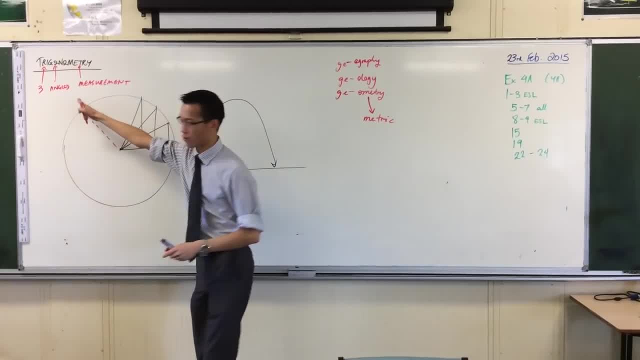 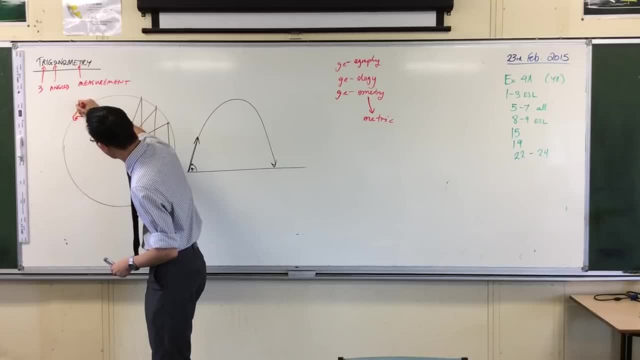 I've got my um, I've got my string holding something to a center of motion. there's my finger in the middle, right, And then you've got the keys flying around there, right? That's a beautiful diagram, okay. 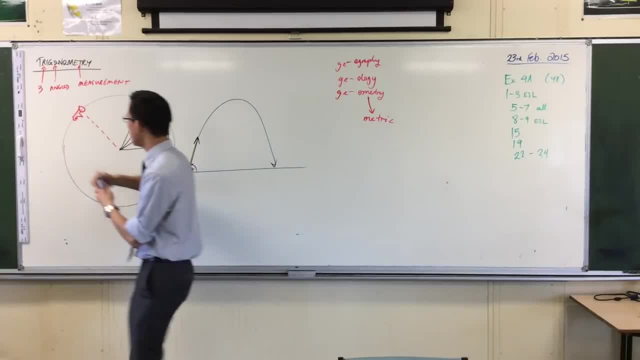 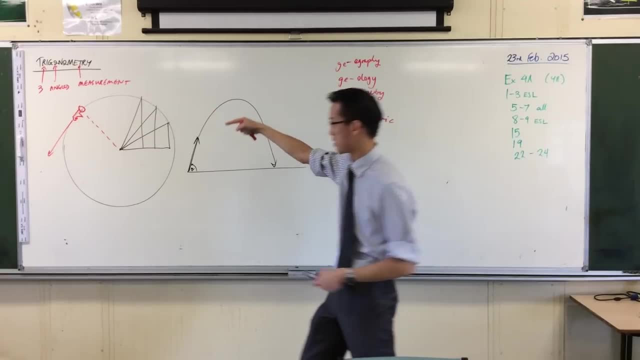 Now have a look at that thing. What's it doing? It's going around the circle and its motion is described by that line there, right? So it's. it's constantly going around. If I get to here, it's going to be going that way. 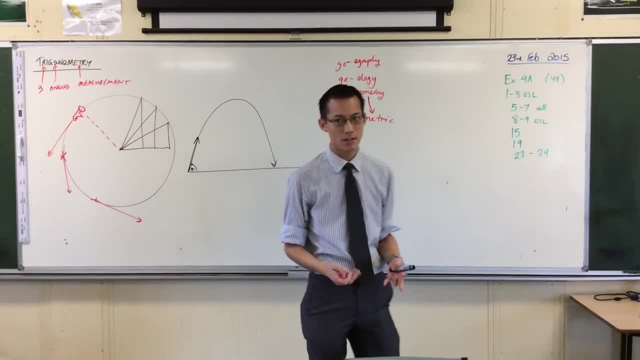 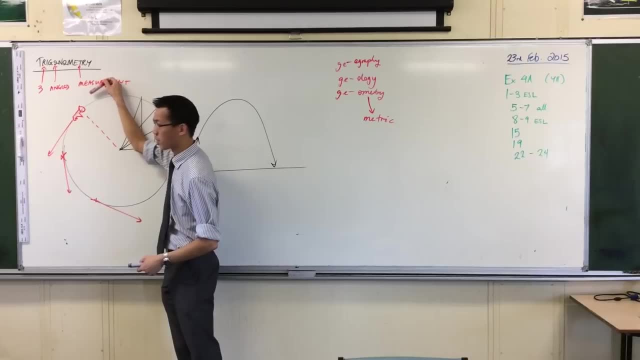 If I get to here. it's going that way. Each of these lines is a tangent. okay, Now what's going on here? all of these different angles of motion, right, We compare things, uh like, uh, what's this called? 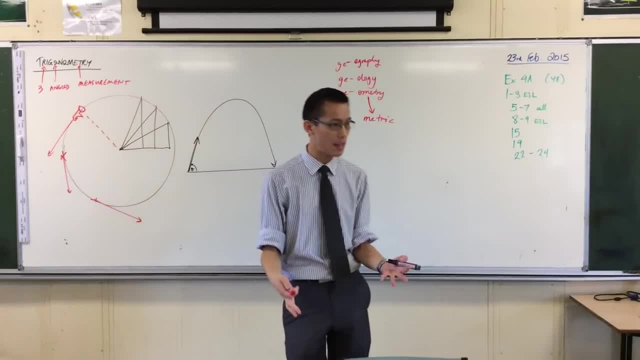 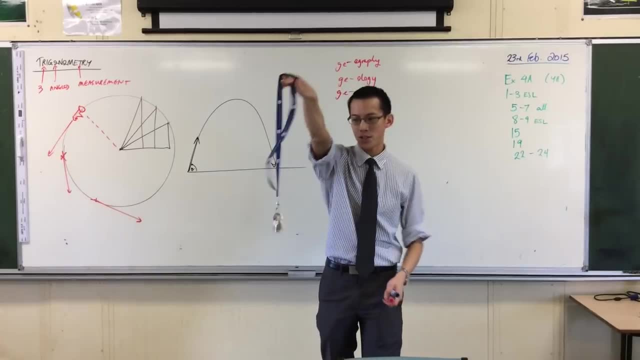 Linear velocity versus angular velocity, all of these types of things, right? They're all built of these things. triangles, right? So, despite the fact that you know where's the triangle in this thing when I spin it around, right?